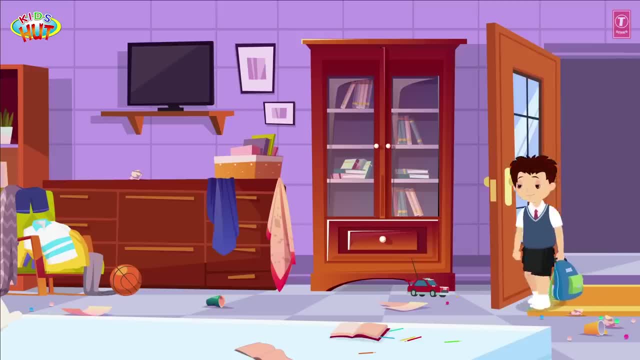 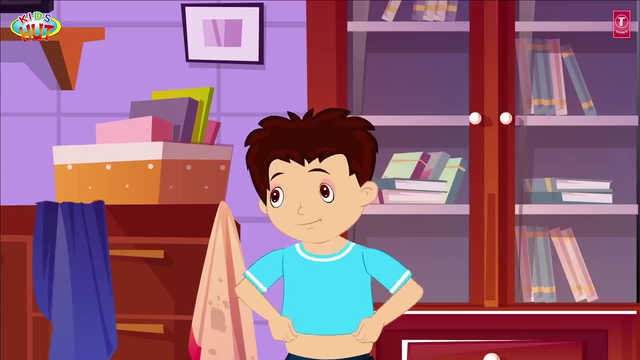 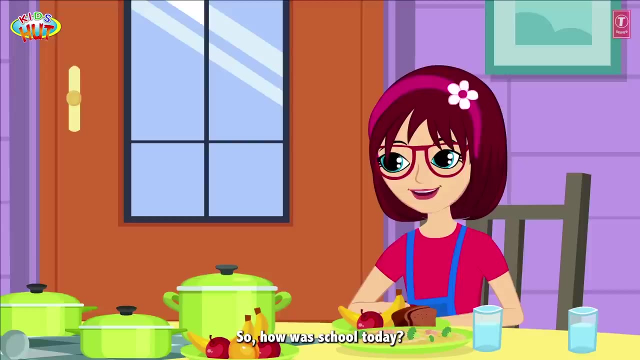 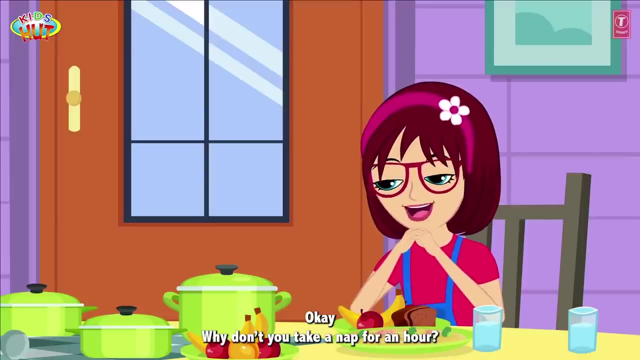 Alright, Tia, Here we have some beans for you. Thanks, Tia. So how was school today? It was good, but I feel a little tired after the hockey match. Okay, why don't you take a nap for an hour? 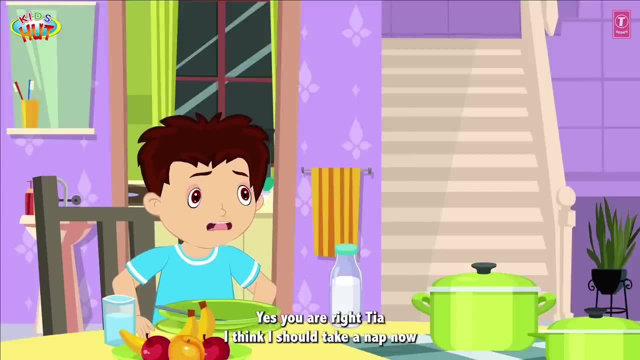 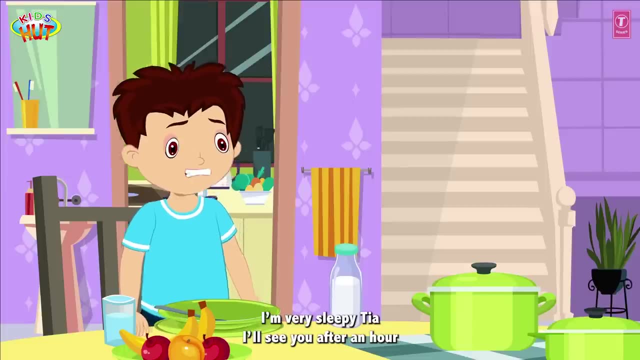 Yes, you're right, Tia. I think I should take a nap now. Tofu, please keep your plate in the kitchen. I'm very sleepy, Tia, I'll see you after an hour. What's wrong with this boy? 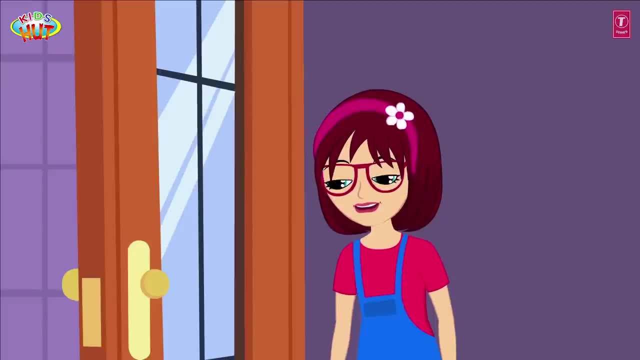 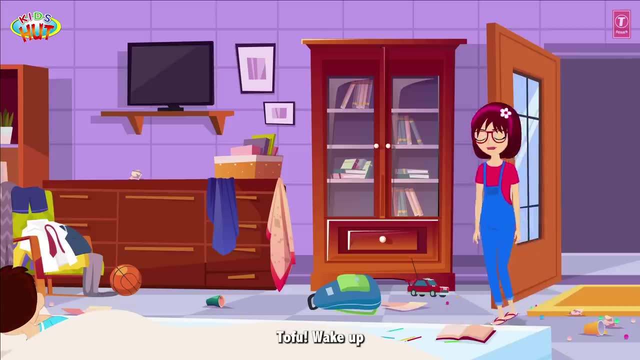 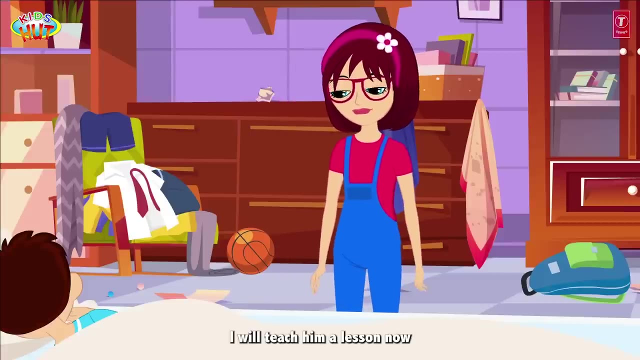 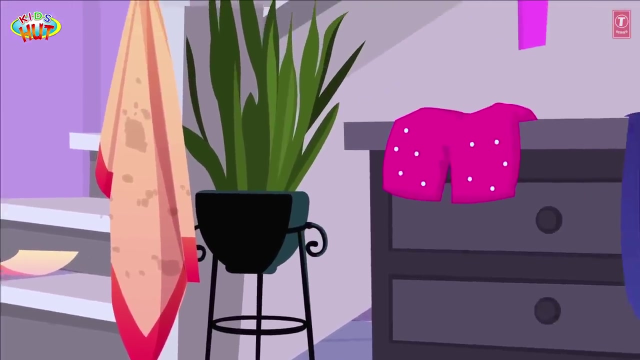 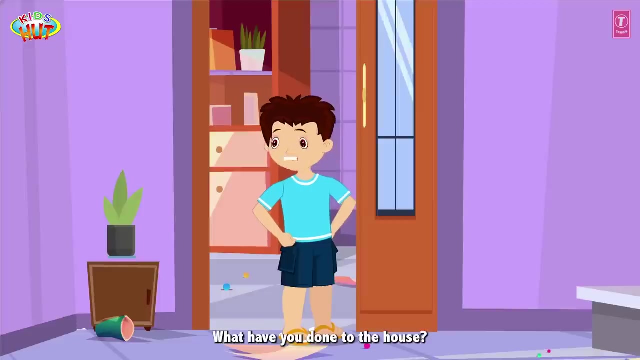 Tofu, wake up. Let me sleep for five minutes more, Tia. Okay enough, I will teach him a lesson now. Oh my God, Tia, I'm so sleepy, I'm so sleepy. What have you done to the house? 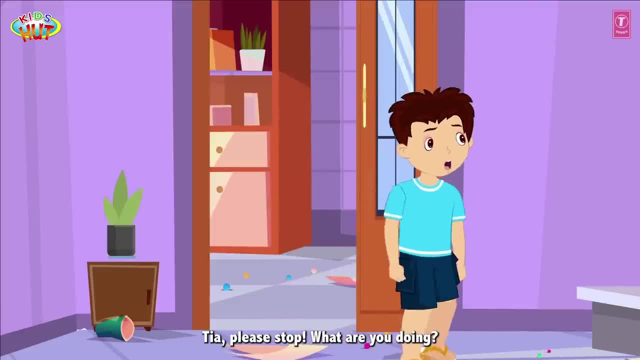 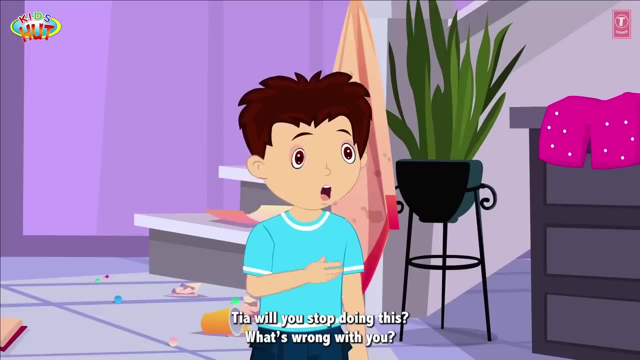 What a mess, Tia. please stop What are you doing, Tia? Yes, Tofu, What is it? Tia, will you stop doing this? What's wrong with you? You are doing the same thing too. 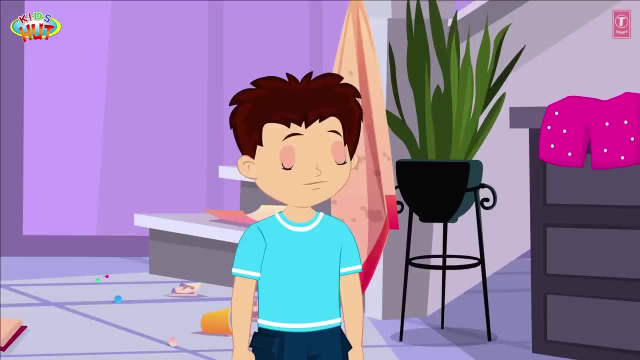 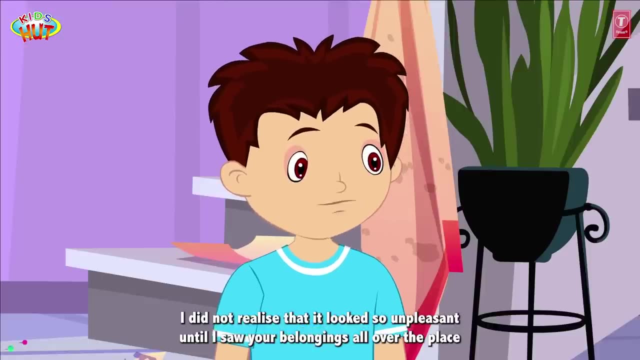 Look at your room. It's an absolute mess. Uh, I'm sorry. I did not realize that it looked so unpleasant until I saw your belongings all over the place. It looks so messy and unorganized. I will keep my things in place now. 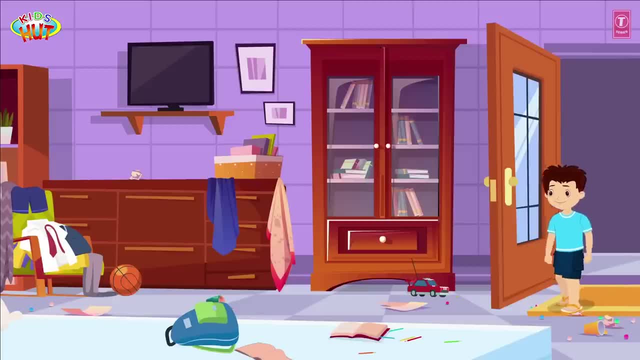 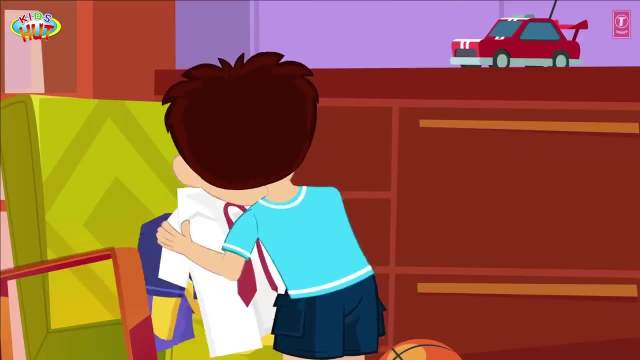 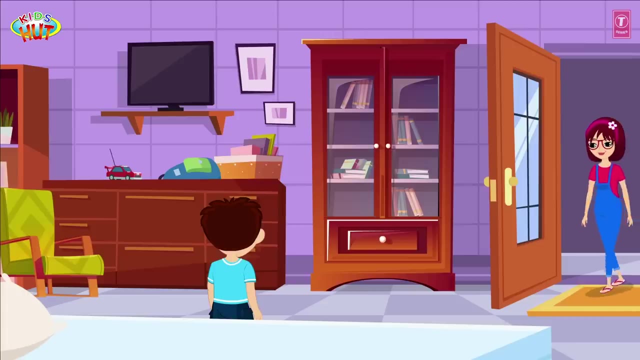 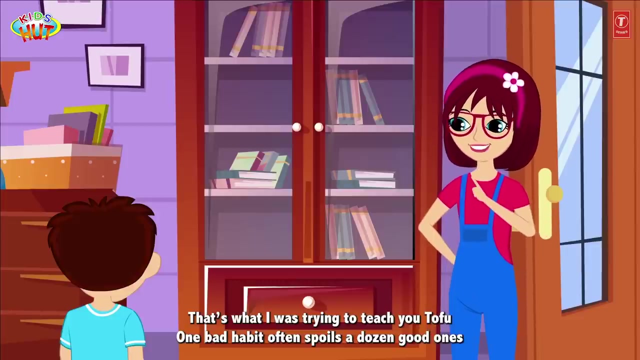 I will keep my things in place now. That's what I was trying to teach you: Tofu. One bad habit often spoils a dozen good ones. That's what I was trying to teach you: Tofu. One bad habit often spoils a dozen good ones. 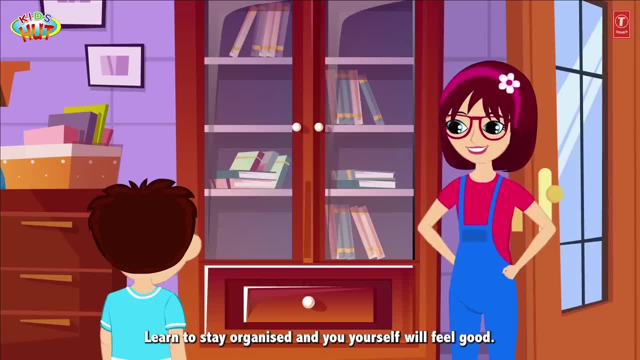 That's what I was trying to teach you, Tofu. Learn to stay organized, and you yourself will feel good. Apart from that, you can adopt small good habits, like holding the door open for someone sneezing with your mouth covered.